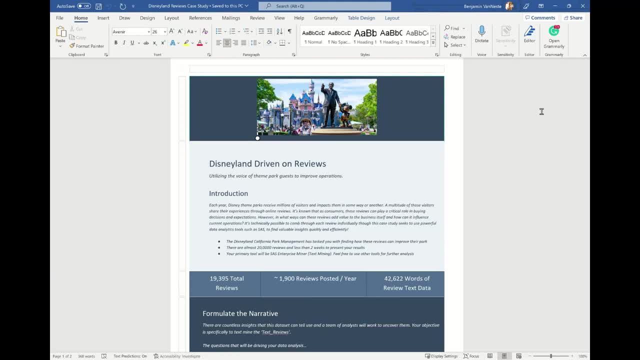 trying to just recommend business strategies based off of what people are saying about the parks and how they're feeling about it. So the primary tool we're going to be using for this is the good old SAS Enterprise Miner, because they have a few text mining tools in there. So, yeah, we can just go. 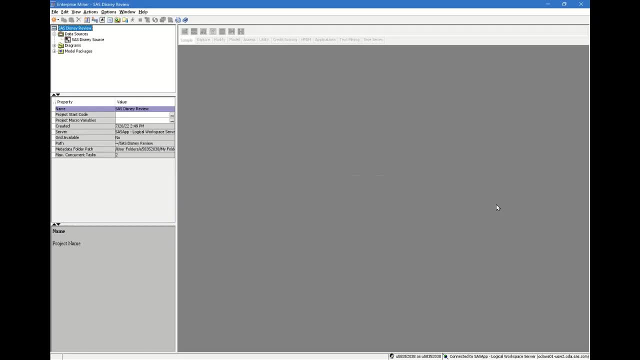 ahead and do that, So yeah, so we'll start. You're going to want to make sure you have the right file for this, because SAS is pretty particular with how it reads the data, So I had to mess with this a lot, So just make sure that you're using the data source that's included on the case study document. 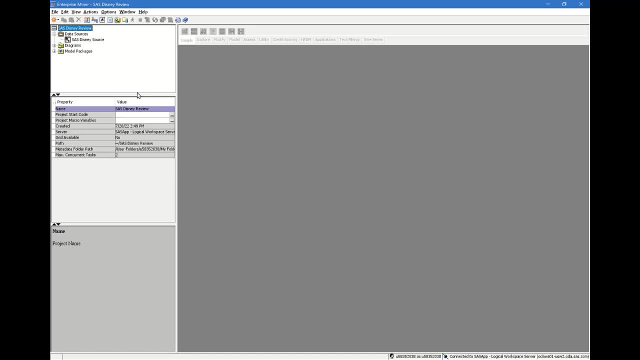 or hopefully I can just put it on the discussion board. Yeah, it's going to be the SAST DL California, the Excel version of it too, because even if it's CSV, then it still doesn't know what it's doing. So try and make sure you have the right data set. 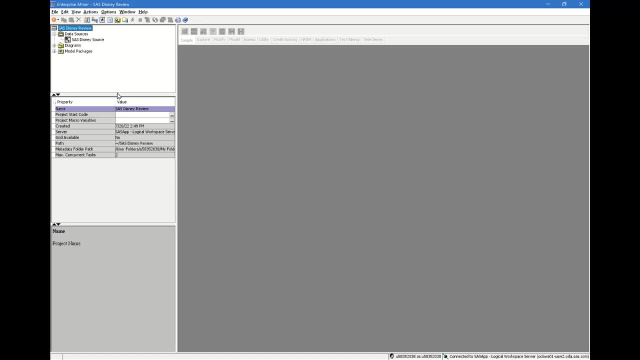 for this project. And then, yeah, you're going to be using the file import node and doing all that to get the data set into Enterprise Miner And so, yeah, as long as all that's ready, then from there we would create a file import. 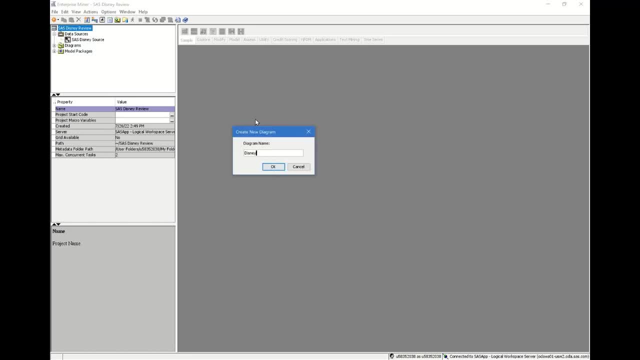 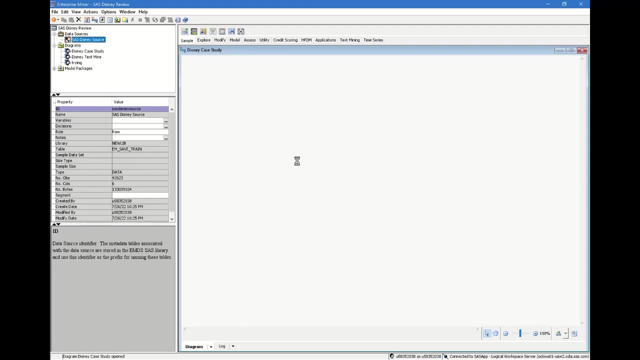 A new diagram- we can call this the Disney case study- And then we'll go ahead right away and throw the data set in there. And then what you're going to do? real quick. we don't have to mess too much with the defaults that are. 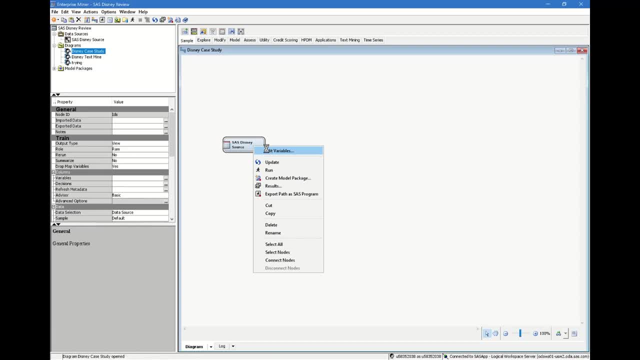 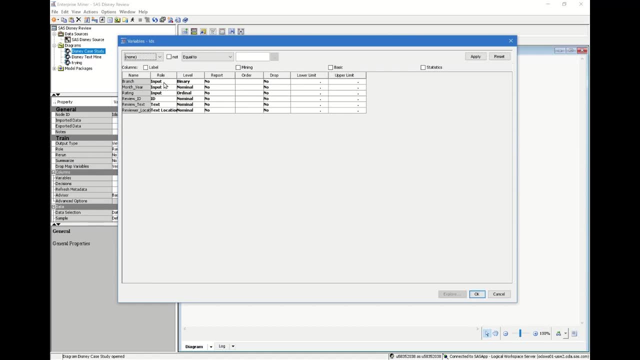 going to be in here, but you are going to want to change the variables. That's very important. Otherwise again, yeah, it'll just be all messed up as you go through. So the branch this can just be rejected. That's irrelevant. 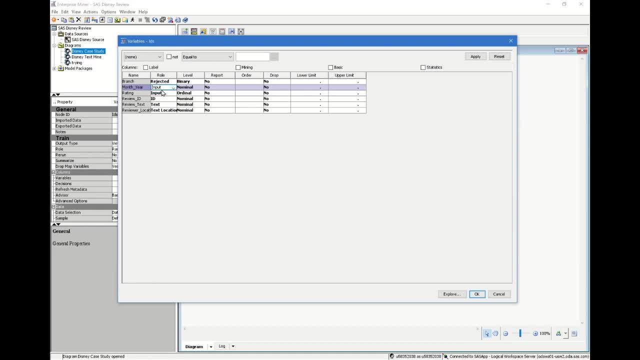 The rest for month and year is going to be an input at nominal Rating is going to be our target and rating and- sorry, rating and review text is going to be our- really the only ones that we really use. So, yeah, we're going to have that set at ordinal as well. 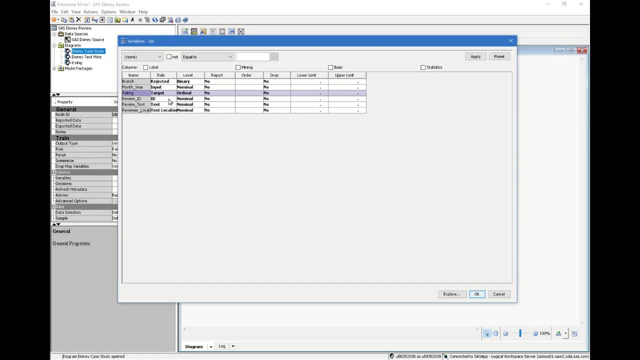 Review ID is ID and nominal as well. Actually, we can change that to ordinal, Not that it should matter, but text is going to be make sure it's at text and nominal and then text location: Yeah, so that everything else looks good to go. 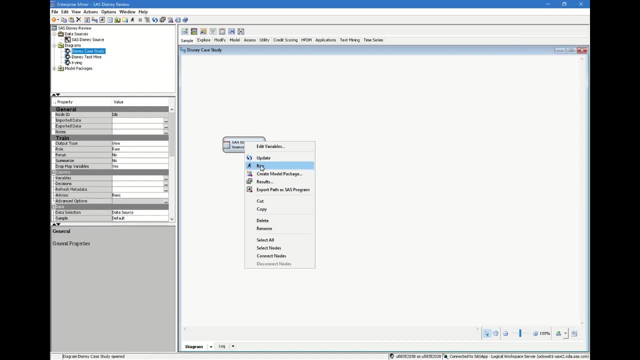 You can click OK and then we'll run that node. I don't know if we really need to do this, but yeah, we can just run it. And then the next step we're going to end up doing is the first thing You really do in almost any with any text mining- I guess in this application is you start out with text parsing. 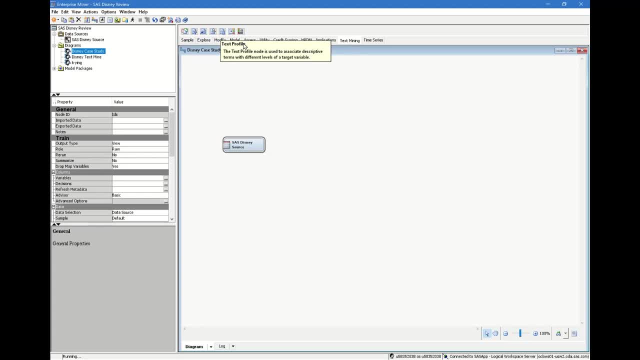 So we can grab that from the top and make sure you go in the text mining tools up here- It's going to be the one with the magnifying glass- and just put that in there. You can connect them and I don't believe we need to change any of these defaults. 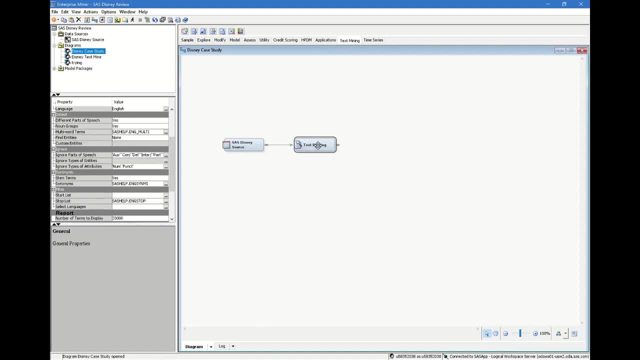 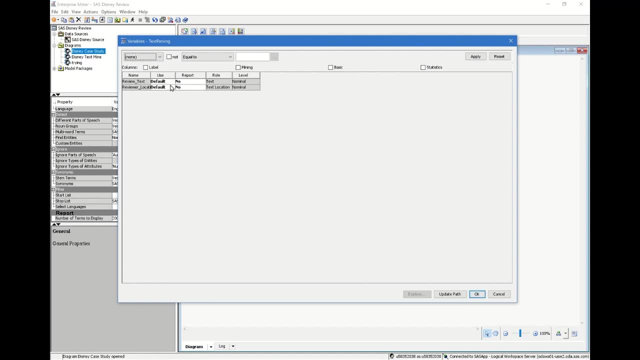 So you can just run that as is actually and just do make sure, I guess, that the variables are Still right, because it likes to change them. So, yeah, actually for this. yeah, we do have to change it. 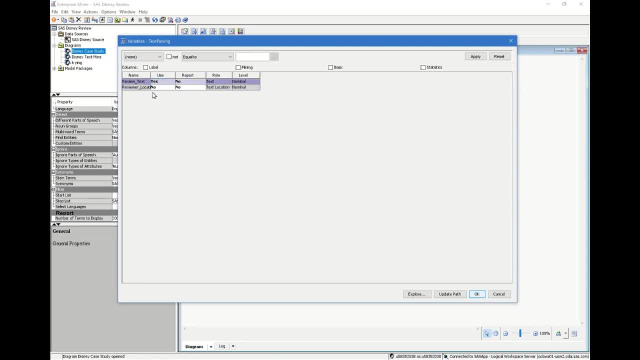 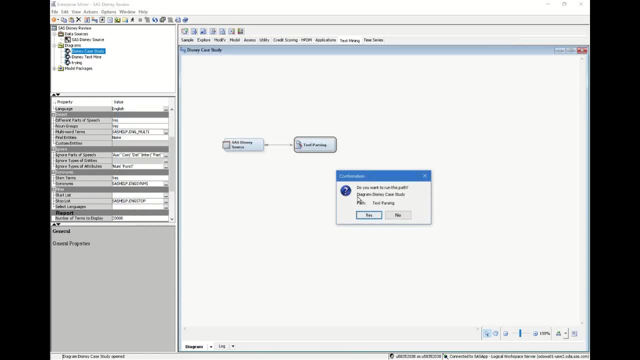 We're going to change that to know, because that's going to be irrelevant, and then review text to yes and make sure that's good And then we can run it. if yeah, if you try to let it see if it can understand the review location, it just doesn't. 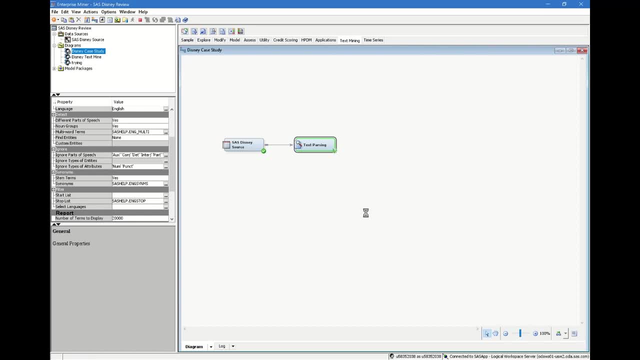 So definitely do that so you don't trip up with that. But yeah, so this node is basically going to Prep our data for the analysis and the insights that it's going to give us later on. It just takes all that raw text data that's in all of the reviews, which is just thousands and thousands of words. 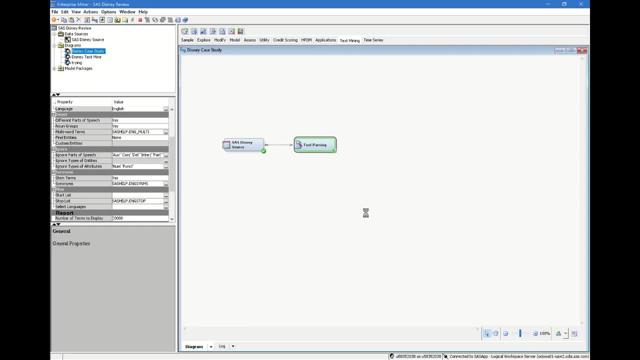 And then it's going to tell us, start to form associations in them and give us terms that are most common. And, yeah, it provides a few valuable insights, but nothing really too special. So once that's done running, we can check the results for it real quick. 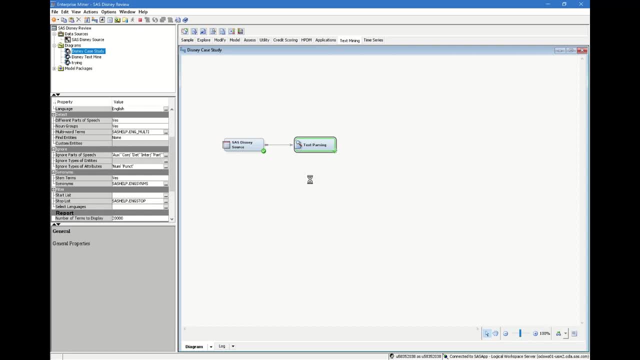 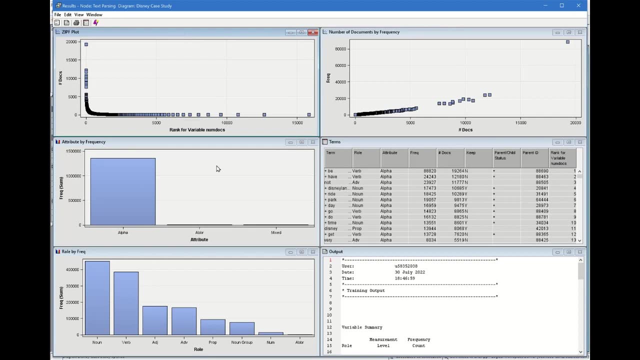 But yeah, you won't really find anything to eye opening until after this step. Awesome. So now we have a results screen here. So, yeah, this kind of just tells you how many noun verbs it tells us, tells you what types of words I guess are. the types of words are in there. 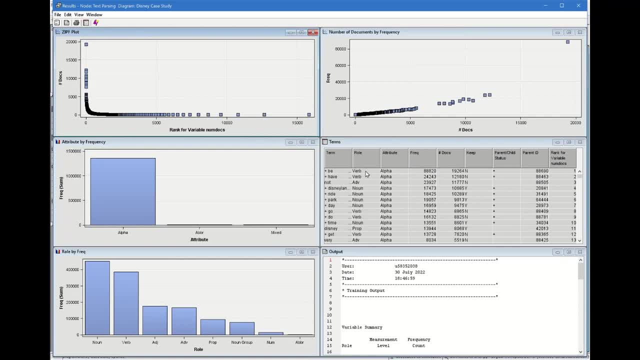 And then this chart here, this table, tells you how Often certain words come in. and then it also starts to group terms together. So something like ride is going to be grouped. It's counts anything Any time the, the parsing finds the word ride. it's going to group it with things like ride or rides, or maybe even riding. 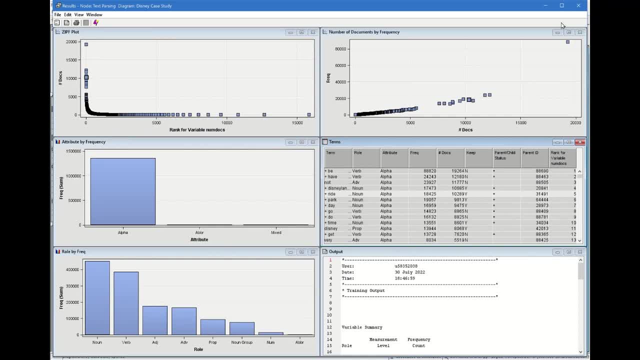 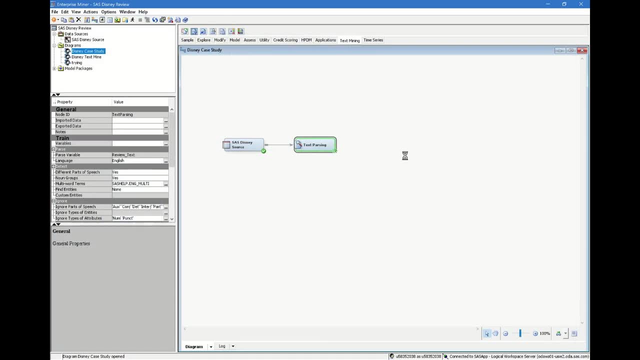 I don't know why it's not opening, but that's basically what it does. So, yeah, we can close out of that, And then our next thing is going to be a text filter, So we'll throw that in here, Connect that and don't mind this, that my SAS Enterprise Miner doesn't ever do these, right. 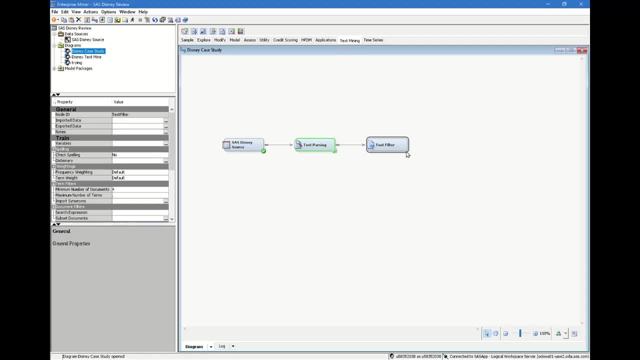 It just does its own thing. So in here we don't have to change any of the settings, so we'll just use the defaults. We'll run that. OK, it looks like that's all done now, So we can Check out the results of that real quick. 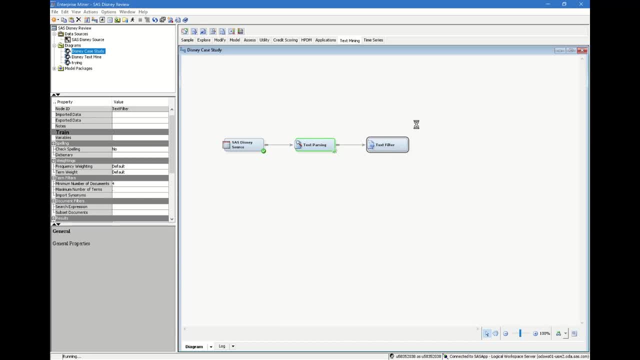 Basically this node is going to group similar terms together and then decides which terms it should keep or drop. And yeah, basically kind of figure out figures, tries to figure out which terms are going to be valuable or invaluable for our future or further analysis. 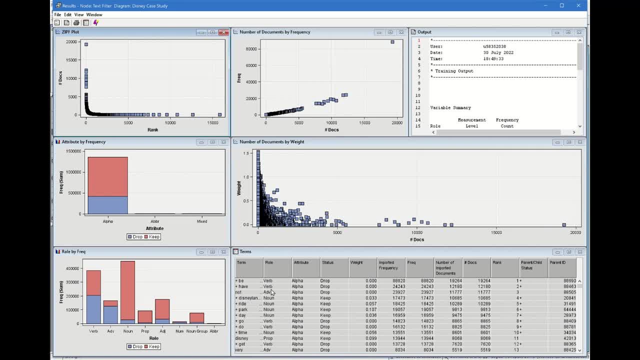 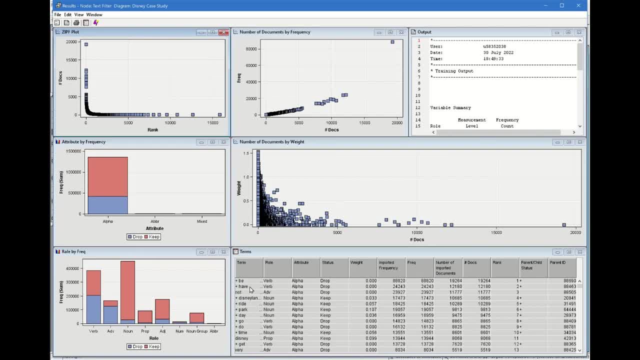 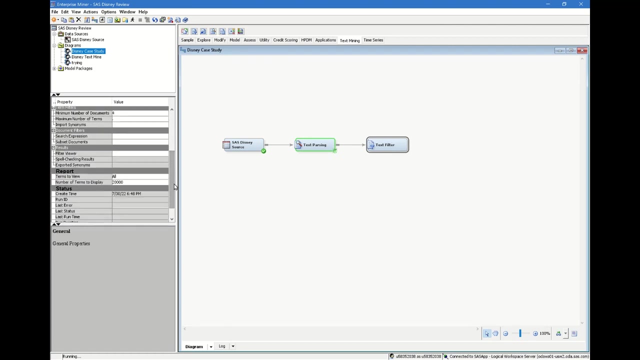 Yeah, Yeah, Yeah. These just kind of show you what's being dropped and kept in there. The more helpful thing that you can find in here is if you close out the results and then you'll go down to here and go into the filter. viewer of the results. 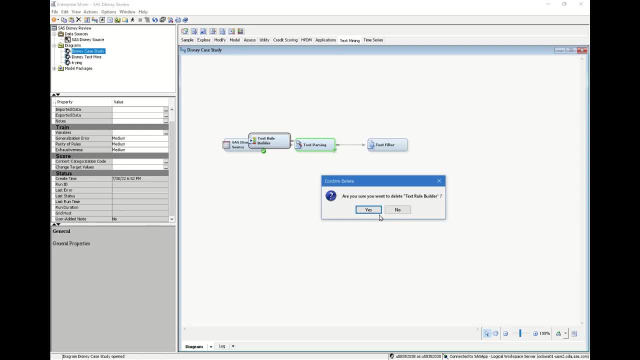 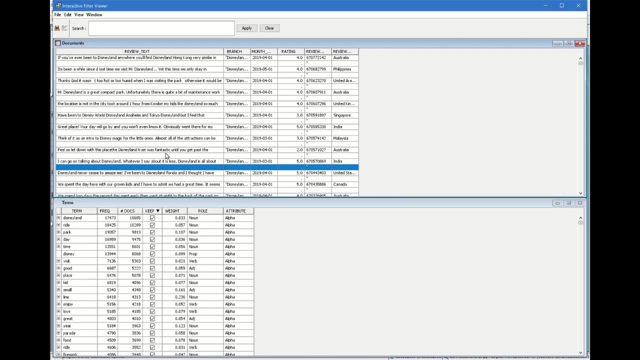 I have to do this for the to actually work. So yeah, you'll click it. go down to results, click the little semi-colon thing or not semi-colon, the dots, whatever- in filter viewer. Okay, so now that we have that, 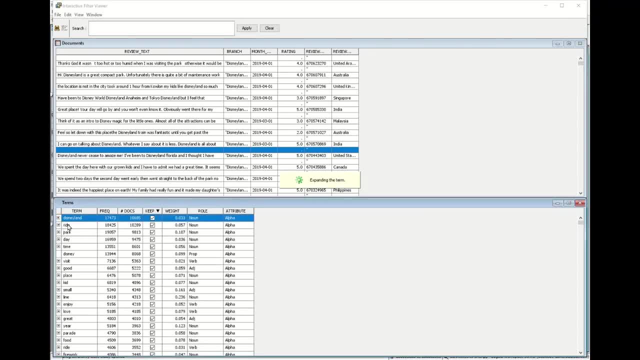 here's where you can actually expand the term and see what's in there. So just Disneyland and Disneyland, that makes sense to group those together, What we can do. so here's the word love, like let's see, we can try and maybe see. okay, what are people talking about? about things. 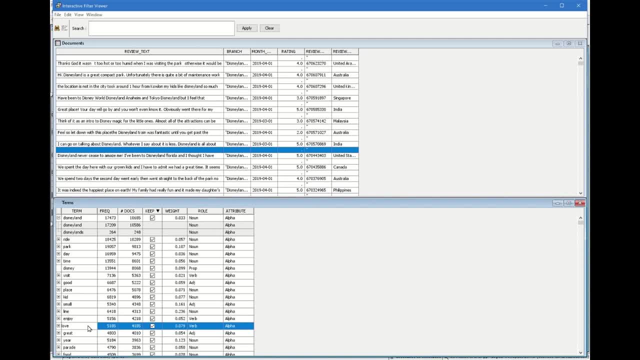 that they love. So you can view the concept link and right-click it and click yeah, view concept links and probably like 30 minutes later, open. there it is, And so this will just give you words that are closely grouped and closely related with it. So we have things like: princess stay. 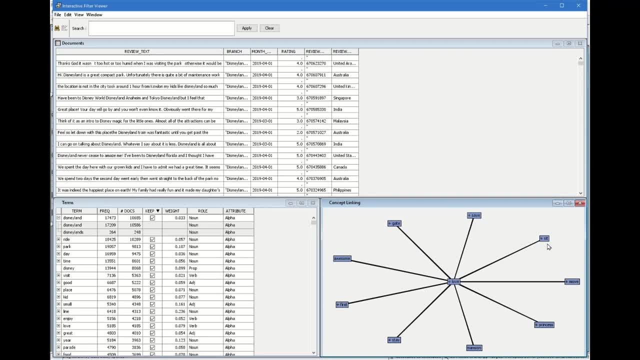 mansion first gate sit and these might be different Because it likes to do different things all the time. But we can see like, okay, maybe is there specific princesses that are mentioned in that, people that the guests love that they talk. 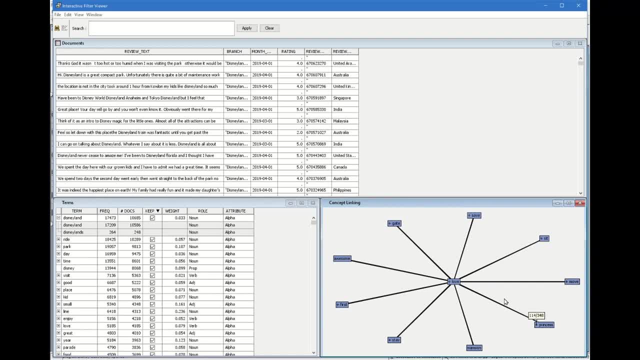 about. So you can double-click that and then, after it freezes for a while, and yeah, there we go. So Cinderella has to be probably a big one, and then it's good it's they get to meet them. 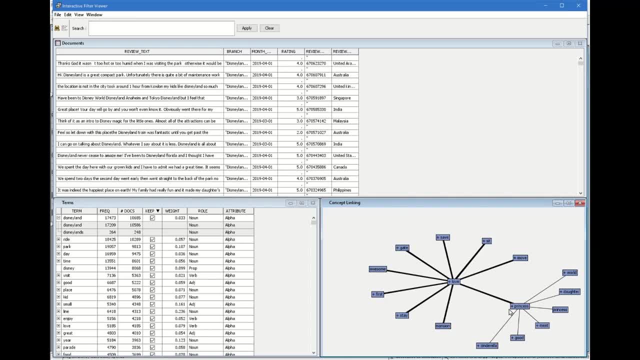 so they like to actually go see them rather than maybe just seeing them in a parade or in a show. And then daughter obviously is, yeah, not too surprising. So you can dig into this even more and more And you can start to find some good insights from that, of terms that are just 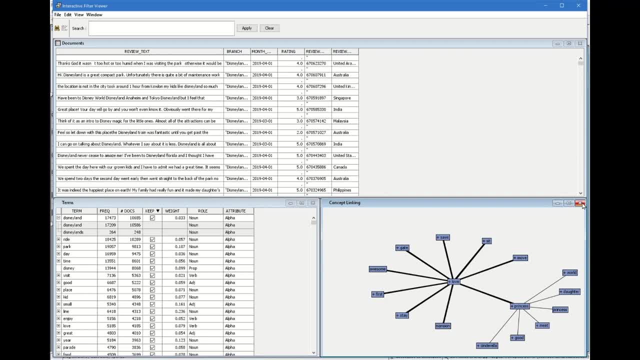 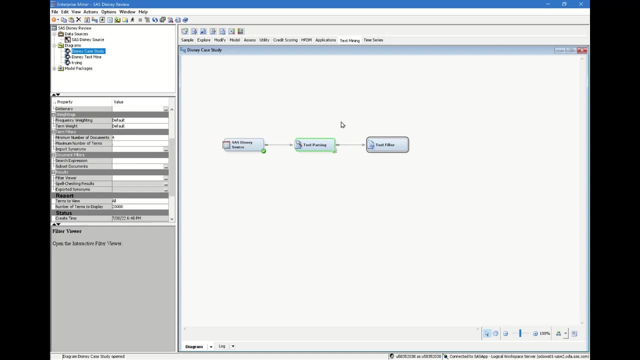 yeah, commonly mentioned, and what kind of. you can even see the weight that they play and how important they are. So we can close out of that. and then now we can move on to the slightly more exciting one: nodes- this will be the text, rule builders the next one, and then we're. 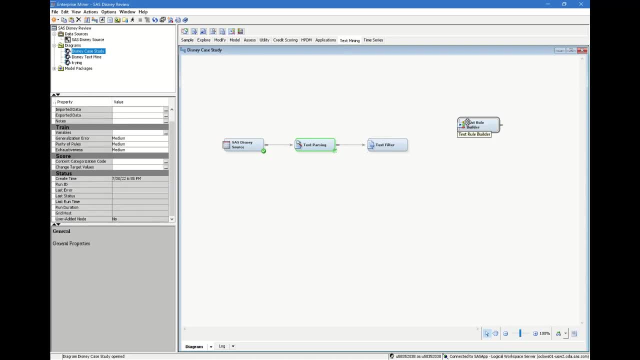 gonna split this text filter up into so you can just put it there and don't need to make any changes for that one either. we'll run it. look for any of these nodes. feel free to kind of make your own changes to any of it, really, if you feel. 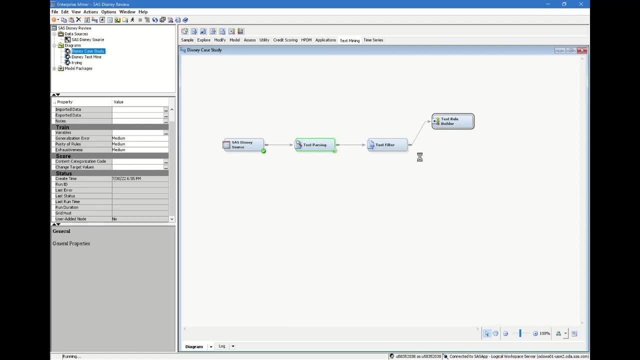 like you might be able to. I'm sure there's a lot that could be better about this entire process, so if you think you can find something better than definitely just do it. okay, now this is all run. I just want to check that the variables were right in there. we'll see, hopefully check the results here. 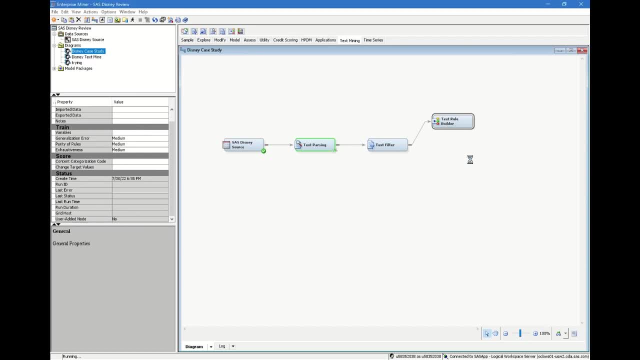 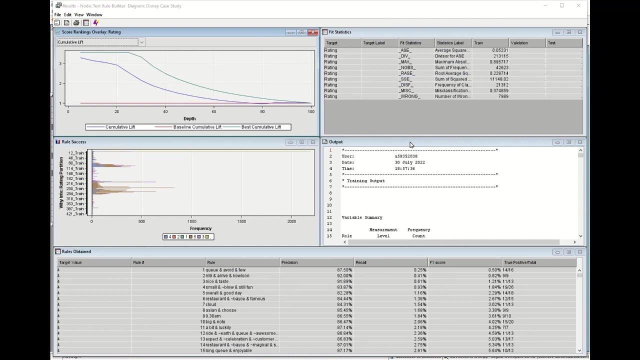 hopefully it was able to do it right. okay, so now that finally booted up, this is what this does: is it's going to finally start to relate all those terms and groupings of terms into the or relate to correlate them with the reviews that we have? so the number of 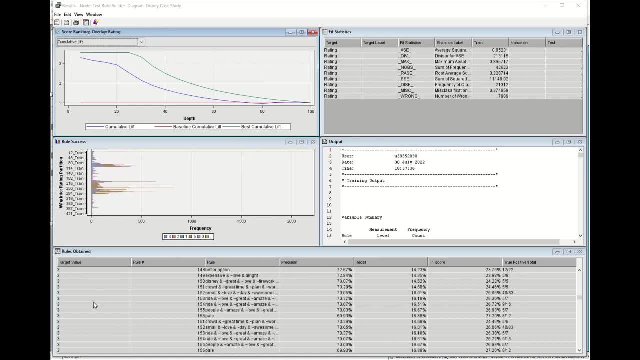 the reviews. so we have, yeah, our five star, two star or one stars and you can start to see all the terrible words with one star reviews. but then if we were to look at the five star- hopefully there's good, better words- they still look pretty bad. perfect, local, small love and rude. okay, interesting life, bad people celebration. 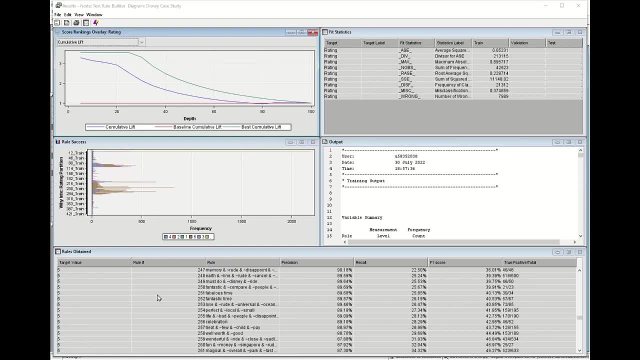 so this is what you would want to look into a good bit more, just to see, okay, and these are, yeah, what's correlated with the heart star reviews, so we have reviews what's correlated with the bad, and you can start to figure out what. what is, yeah, mentioned more so, and it gives you different rules and these like 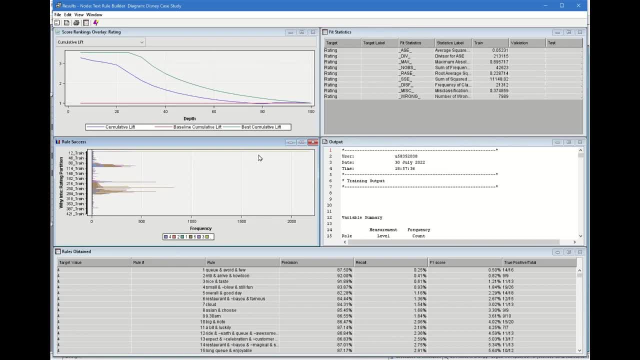 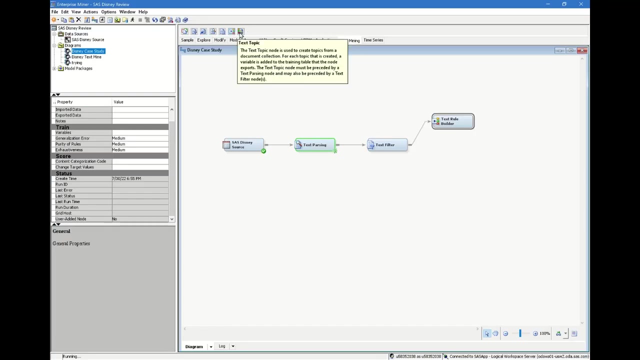 trains and stuff, to try and figure all that out and find, find, find things on your own. it obviously doesn't highlight the majority, but you can just look through and and see. so we'll close that out and then move on to our second to last node. this one is going to be the text topic. roll that in there. 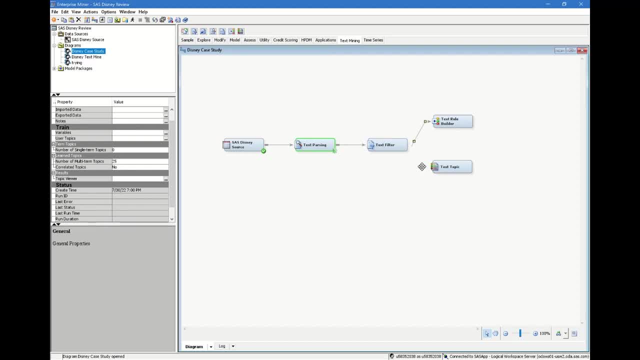 connects go and then for this one, I think we- so we're gonna change this- is gonna just just just just just group those words into topics, basically, and try and label what people are talking about. I like to see the single term ones, because this it just takes the single words or terms that are talked about most and shows you those as 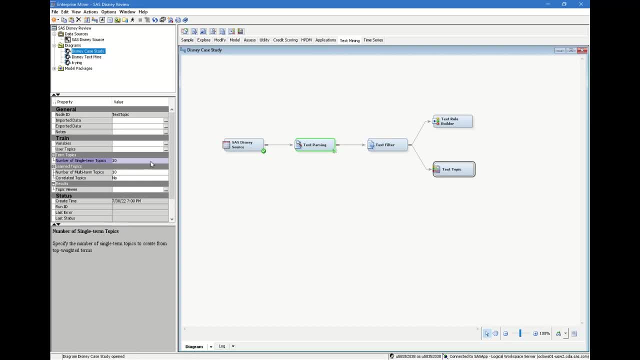 well, and then the other 10 multi term can show you that as well. so 10 and 10, but if you want to make it more and see more of them, if you want to see less, um, just change that up as you want. it got the results for it, and here's this one. 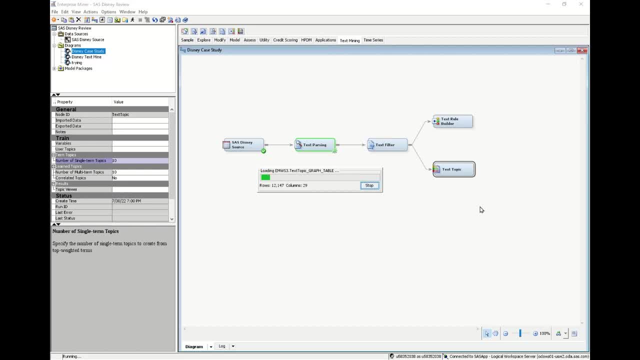 is where I found most of my insights that would be valuable to present. but again for you guys, it might, might be anywhere else and just try and find, honestly, your own things, because that's what makes the whole case study better. it doesn't have to be just one single answer that there's definitely no right. 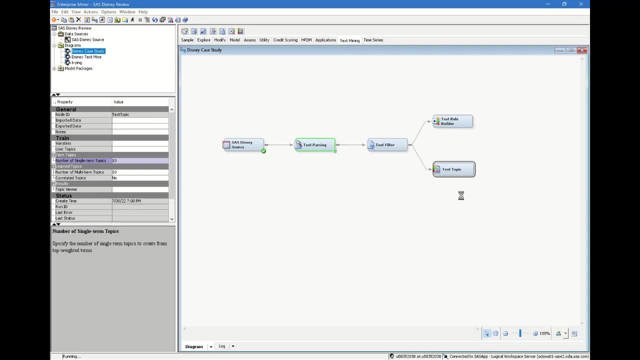 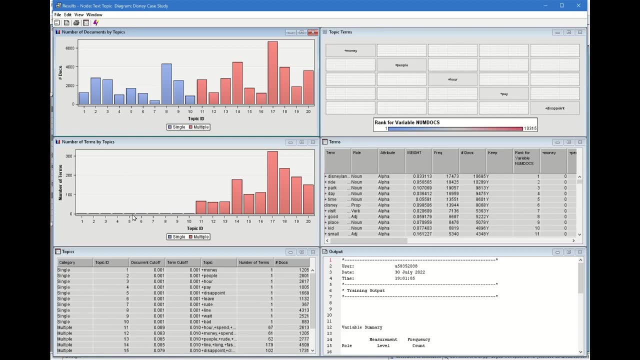 right answer. so, yeah, here's where we have this. okay, wow, yes is different every time. I do it so weird. we have a bunch of the single terms that are mentioned most frequently, so you can. they're sorted by the Docs that they're in. this tells you their frequency or the number of terms as well. that shows you. 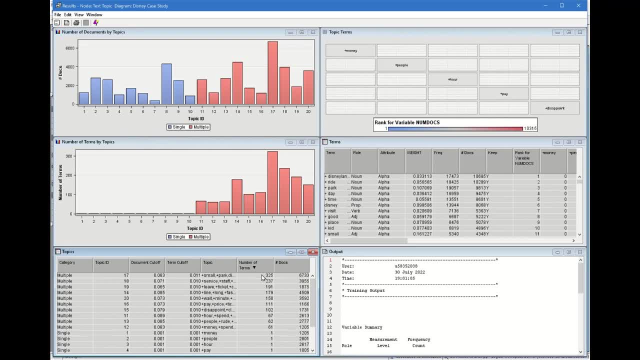 how many terms are in a single topic. so you can kind of expand this to see what's in there. this one's mainly talking about the parks, this one's mainly talking about the lines and maybe the speed or the weights of them. here we're talking about people and then, yeah, you could kind of look into these to see. 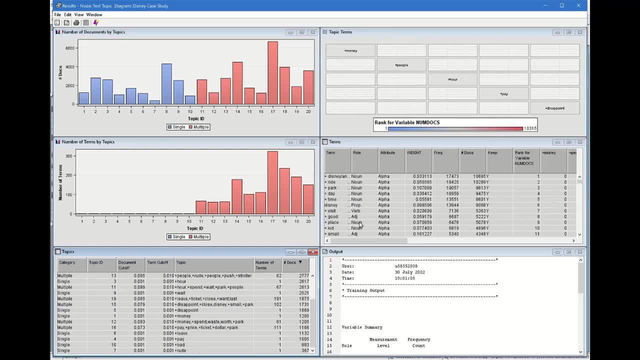 again what people are talking about. and then what I did was looked at some things that were important to me and then, like what I noticed, there is a lot of these most frequent topics- and then, um, like some surprising things i found was like that with lines: um, when i looked at the actual data set, uh, and the reviews that mentioned lines you would think 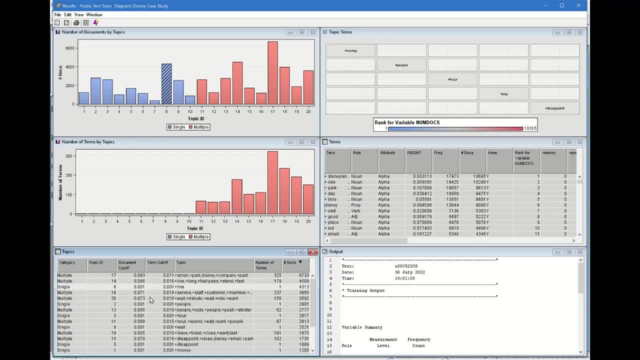 most of those reviews would probably be bad if they're mentioning that, but, um, surprisingly- like with that, it was- most people were speaking highly of the lines and that they weren't too high of weights. so, um, something like that is again valuable to to whoever's running the parks. 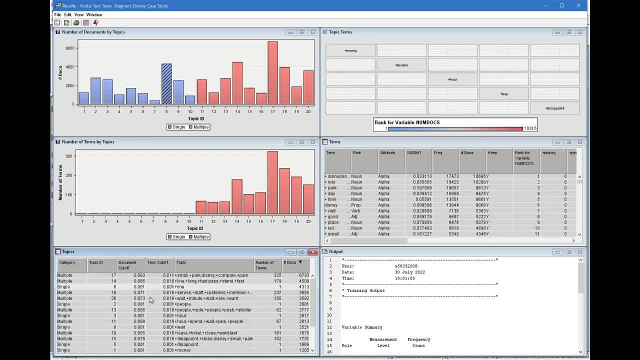 um, and that that's one thing that they're doing well, and so maybe they can focus on that a little less and focus on something more or more on something else, um, or they can, you know, continue to do that, obviously, continue to do that well, um, and find newer improvements if they want to. but 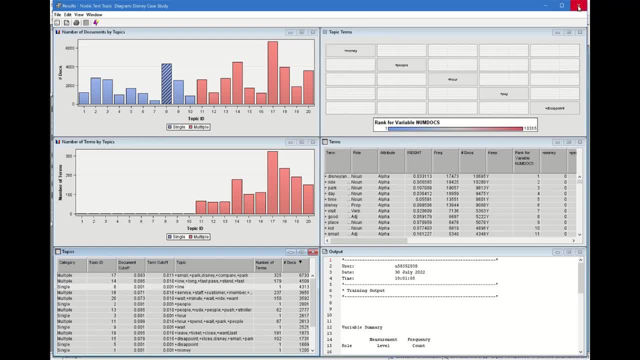 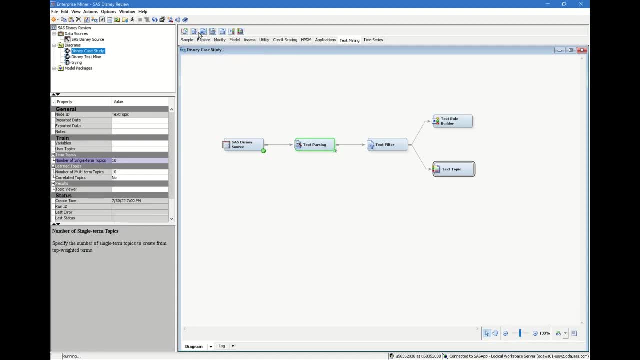 yeah, so that's your text topic node and then, if you want, um, we can throw in the text cluster, um, just kind of complete the whole text mining process. uh, this one isn't totally necessary, but um, again, if, depending on what you're looking for, this might. 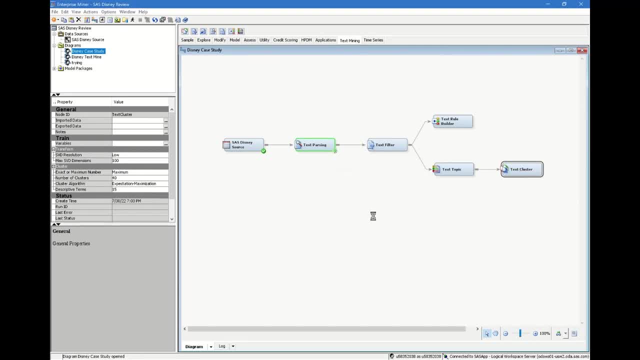 give you the things that you're looking for. um, so it basically just expands on the text topic node and similarly to some of the data mining stuff we did in here- maybe another in the previous courses. uh, this, instead of just like data points, like maybe the numbers and such, 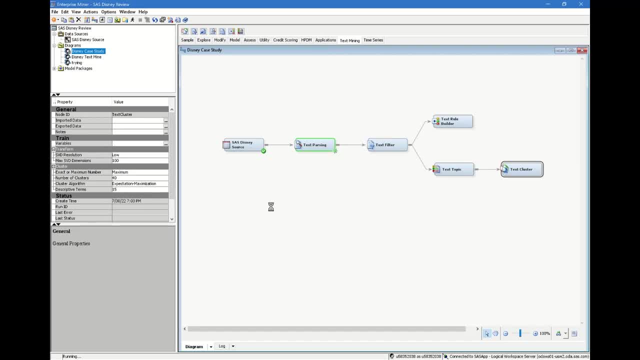 um, it basically takes all those terms and throws them all out on- you know, this is my best explanation of it- but throws them all out on a graph and then um, finds the clusters of them that most closely relate and then puts them in there and then also shows you how closely these groups, um, or kind of. 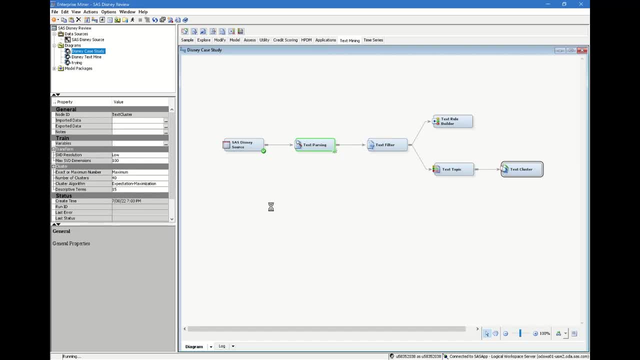 the topics, like we saw before, um, how closely related they are to each other or how far off from each other. so it's somewhat helpful, um, but it definitely takes a little bit more uh, digging into. it doesn't really just tell you things right off the bat. so we can just check out the results for that and then this will. 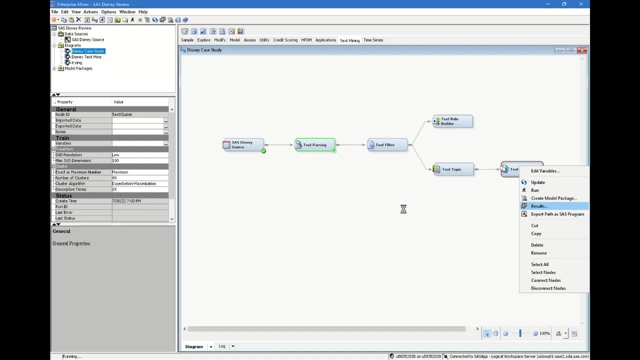 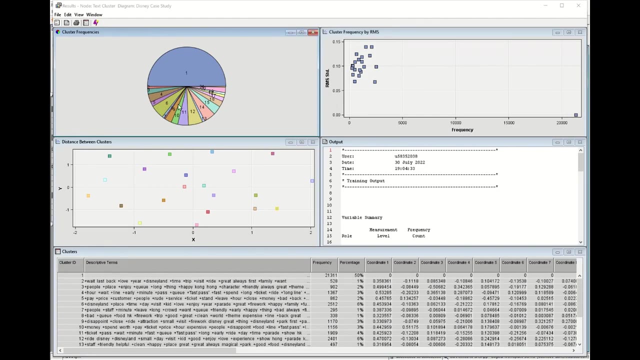 be our last part of it. you made it there. we go um. so yeah, your results are honestly probably going to look different than this, because i don't, i really don't know how i've done this three times. i don't know how i've done this three times. i don't know how i've done this three. 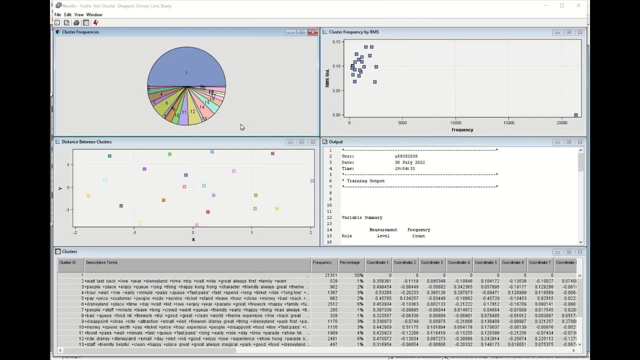 times almost now, and every time they it says uh, ems just changes it up on me. so i honestly don't know how to uh produce the same results that i was getting before. i don't know why it keeps changing. it's kind of has his own personality, i guess, but um, so yeah, this is pretty helpful. i don't even know. 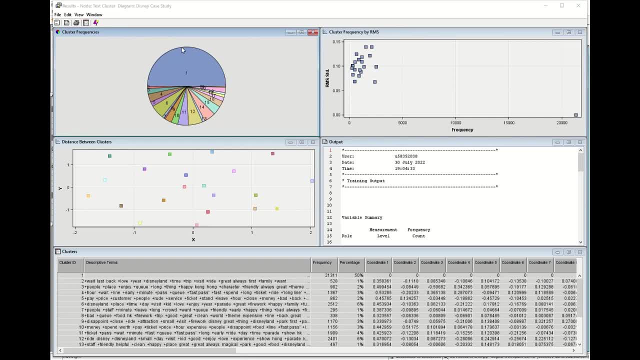 what this first group is. i think this is because it uh read- yeah, that seems right. it read half of the data set as quotation marks, when those, all those rows are invalid. so it's not supposed to do that, to do to sorry to do that. so hopefully you don't see that. um, it didn't. that's the main thing i was. 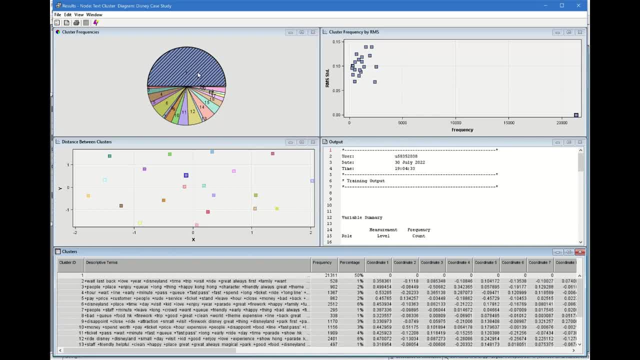 trying to avoid over and over again in the previous uh analysis that i did, but the rest of it is helpful, even though these percentages aren't what they should be. but, um, yeah, you can start to look at uh, all of these groupings, and some of this is really helpful. 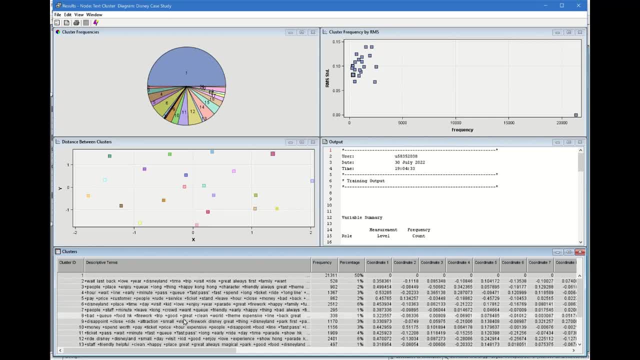 um, because, yeah, it'll typically be uh good words or like positive words, along with maybe things that they liked, um. so here's parade, uh, kid. so it helps, i guess, if they have kids with them. um, clean, um food, good food. so you can start to relate things here and find that, okay, these are. 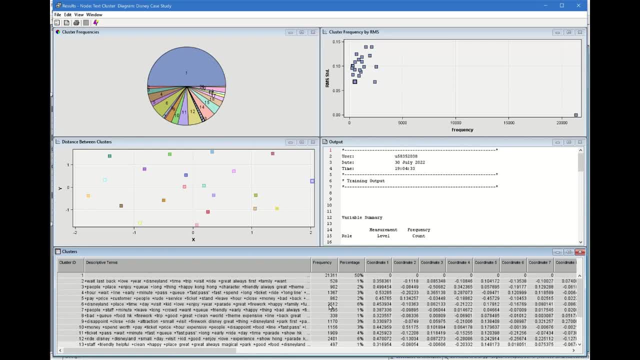 things that are are usually with the things that people are speaking highly of, and then here are the things that people are speaking lowly of. um, so, yeah, that wraps up the entire um yeah process in sas enterprise minor, and then the rest of it is just your um pulling of insights. 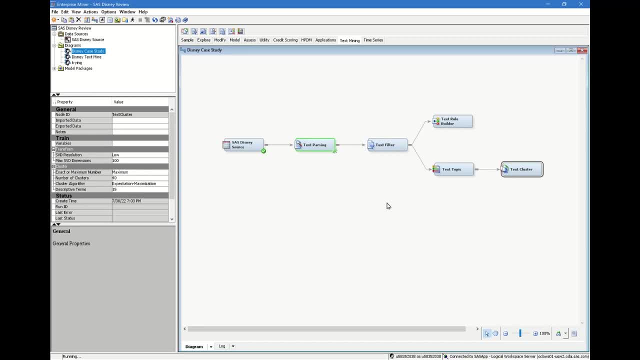 from it. and then again, what? what from this could you tell, like the disneyland california park management? hey, these are some areas you should focus on, these are some areas that are really bad or really good, and then your suggestions for what they could do about it. so, yeah, thanks for following along. i hope that wasn't too confusing. but um, yeah, that is all.